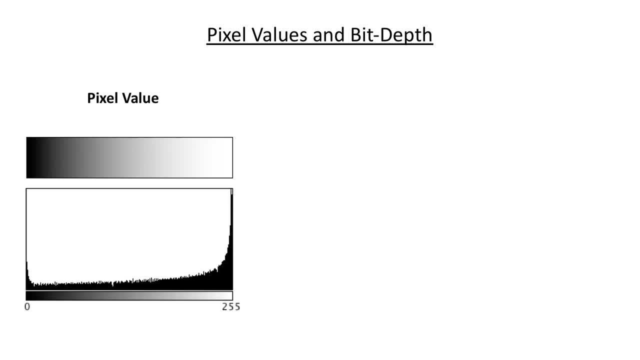 As already mentioned, the grey tone represented by a pixel depends on the value of the pixel, The pixel value and the bit depth of an image. The pixel value, or pixel intensity, is the value of a pixel within a certain range between black and white. For example, we have here an 8 bit image of a gradient between black and white. 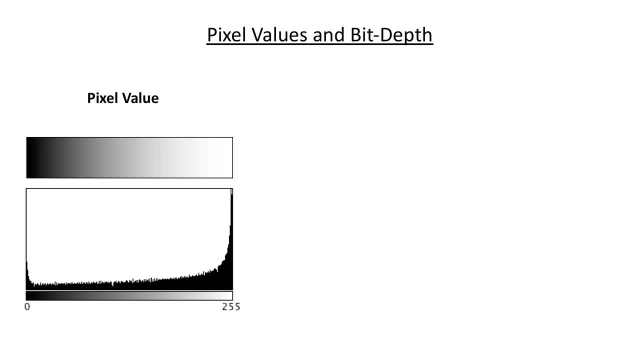 When we look at the histogram below, you can see that the scale is ranging between 0 pure black and 255 pure white. All the 254 steps in between represent the different shades of grey that can be represented by a pixel. Hence the histogram gives us information about the intensity distribution in the range of the pixel depth of all the pixels within an image. 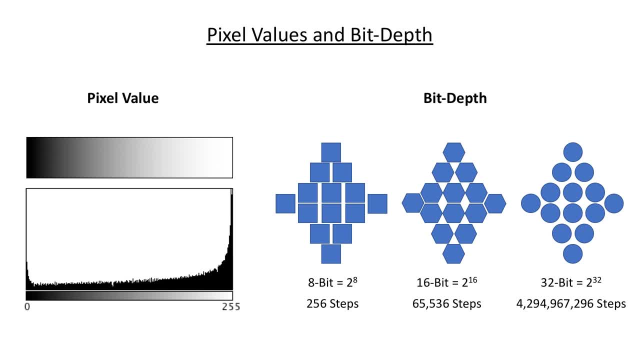 So what's the pixel depth? The pixel depth represents the number of different shades or pixel values in between black and white. So, in other words, when an 8 bit image is like creating a form using squares, a 16 bit image is more like creating the same form using hexagons. 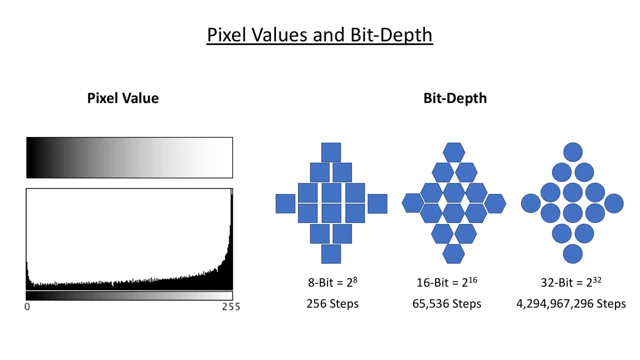 and a 32 bit image more like using circles. In the end, the surface of the form built up by circles will be much smoother compared to the one that was formed by squares. Thus, the higher the bit rate, the more different pixel values or grey tones can be represented. 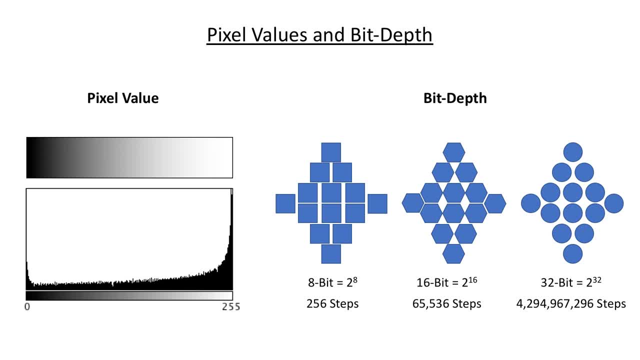 and therefore the information that can be stored in a pixel correlates with the bit depth. However, you should be aware that the actual range of possible values depends on the acquisition equipment. So a 16 bit image obtained using a 12 bit camera will only have 4094 steps between black and white and not the 65534.. 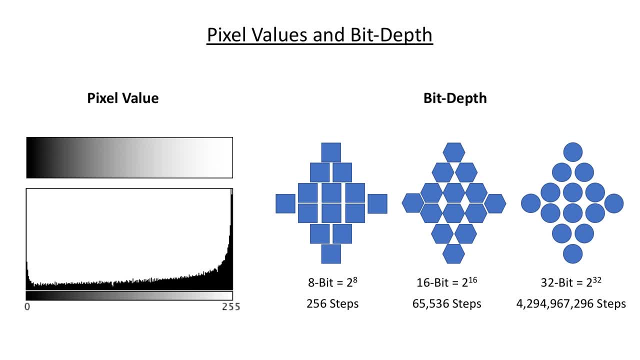 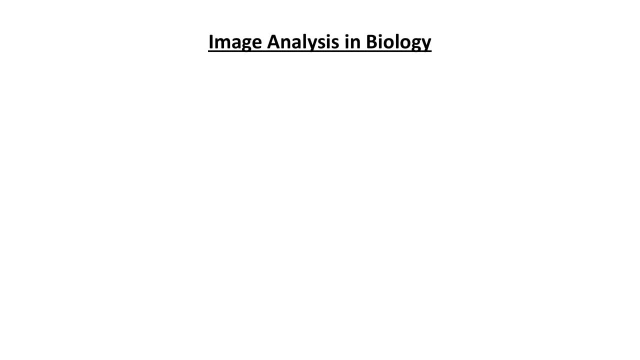 Therefore, the lower bit depth will always dominate, So please keep that in mind. So what is all of this good for? For instance, a biologist will pretty likely work with images- micro or microscopic- that document certain processes, and these images can be quantitatively analyzed. 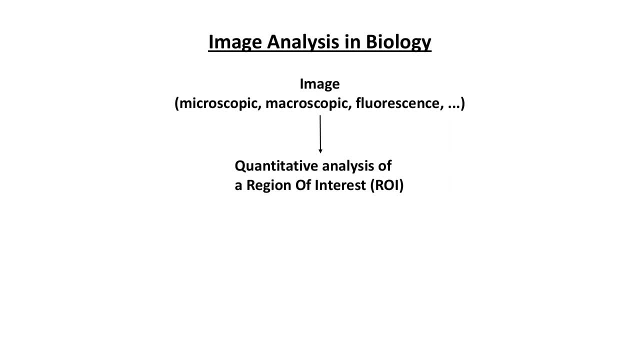 Here the type of analysis can be divided broadly into two different types. On the one hand we have the size analysis. Here the length or the area of a region of interest is measured by counting the number of pixels, and this can be used to determine, for example, cell size, growth, cell migration. 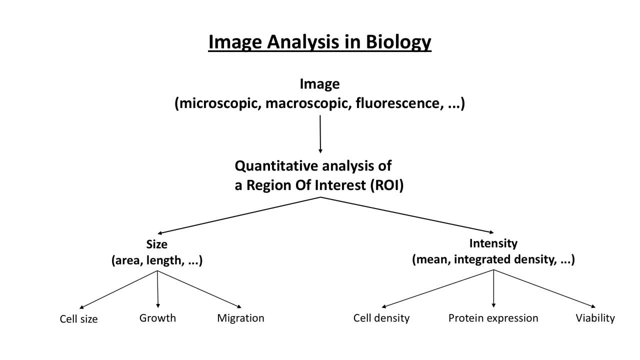 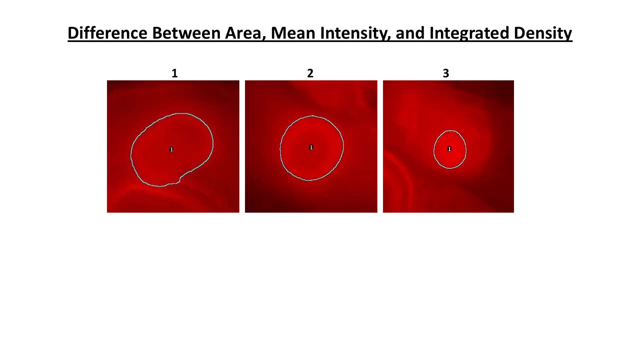 In contrast, the intensity analysis of pixel values as mean intensity or integrated density can be used, for instance, for quantifying cell density, to analyze protein expression or determine tissue viability. Now I am going to explain the difference between the three measurements- area, mean intensity and integrated density- using these three fluorescence images. 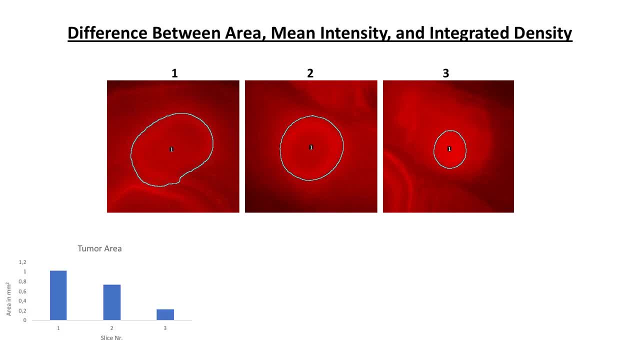 Starting with the area of the region of interest represented by the blue line, You can easily see by eyeballing that the first image has the largest ROI. Next comes the region of interest in the middle image and lastly the one in the image on the right, which is clearly the smallest. 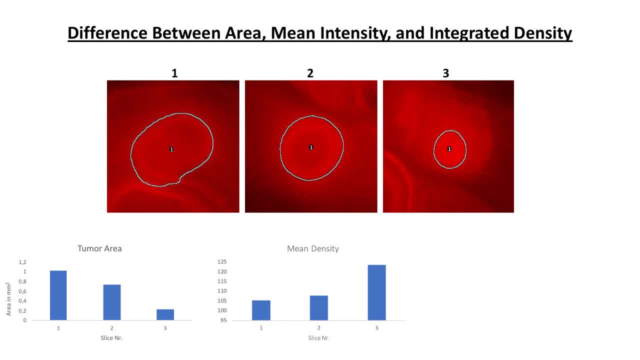 However, when we determine the mean pixel intensity, the right image with the smallest ROI has by far the most intensive red, followed by the ROI in the middle image and finally the ROI in the image on the left with the lowest red intensity. In contrast, the integrated pixel density considers the area of the ROI. 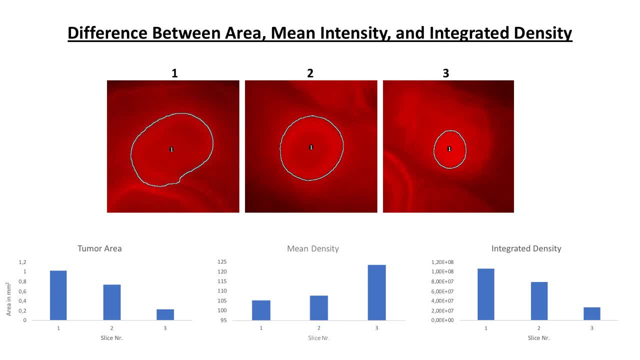 which is why the image on the left, with the largest ROI, has the highest integrated density In twinkly. the ROI with the highest mean pixel intensity has the lowest integrated density, And this should be no surprise, as the integrated density is equivalent to the product of area and mean pixel intensity. 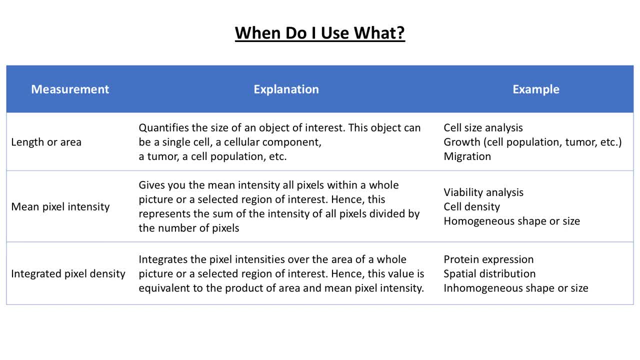 In summary, the length or area of an object of interest is determined by counting the number of pixels and can be used, for example, to analyze cell size growth or migration. The mean pixel intensity, on the other hand, is the mean of all pixel values within an image or a region of interest. 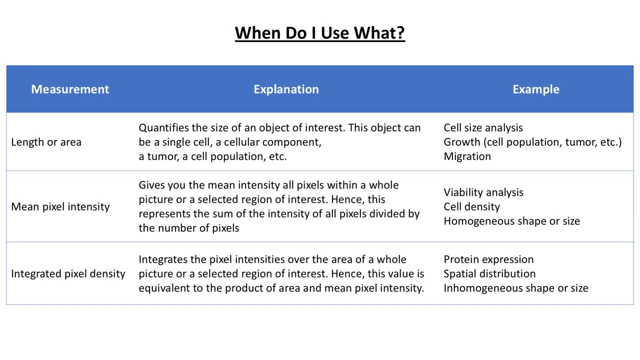 and is usually used for quantification independently of the size or when the size of the ROIs are very similar. Hence mean pixel intensity can be used, for example, to determine tissue viability, cell death or cell density. Finally, the integrated pixel density is determined by integrating the pixel values over the area.